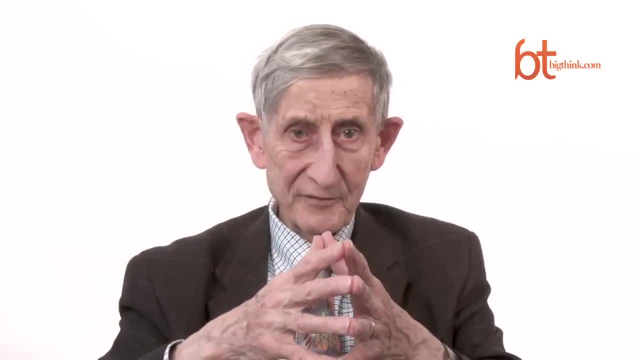 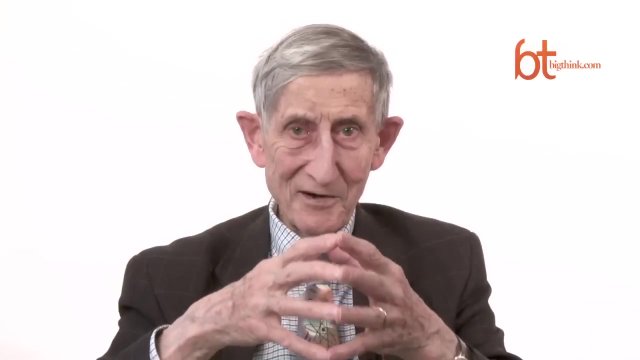 or not, And as far as I'm concerned, it's very foolish to do anything spectacular in that What we should be doing is dealing with the problems in detail. I mean the first thing is we should build dikes around New Orleans. I mean there are simple, practical. 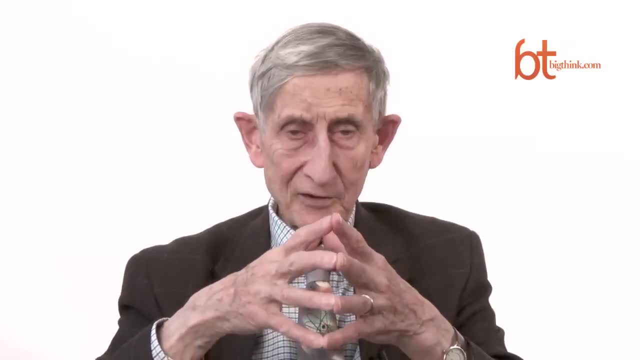 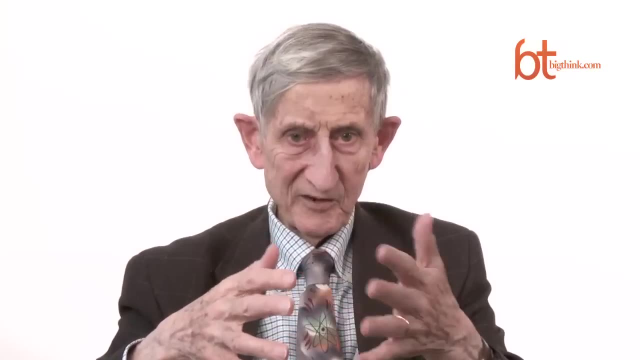 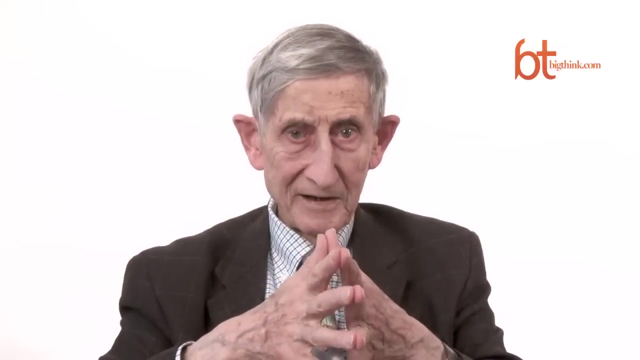 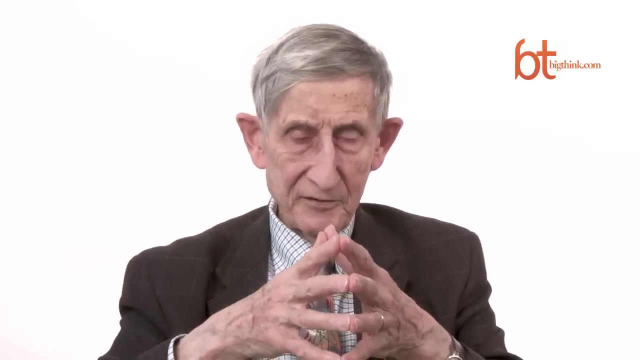 things we can do which really would help, like building dikes around cities which are exposed to hurricanes or tsunamis, And so these kinds of practical measures could be enormously helpful. I mean, we've seen just in the last few months, we've seen two big earthquakes, one in Haiti and one in Chile. 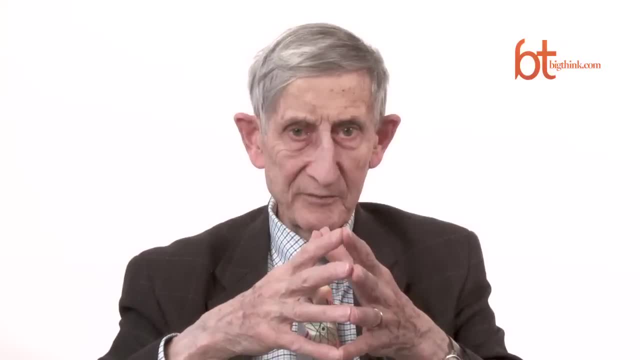 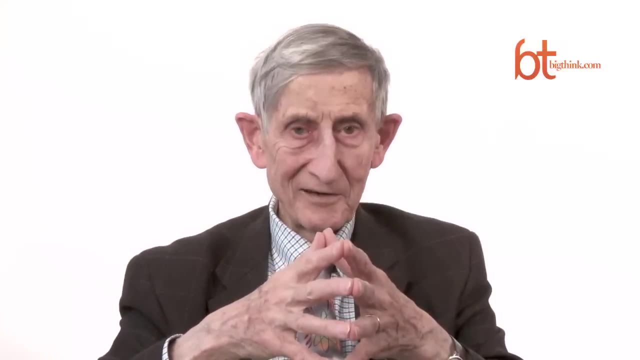 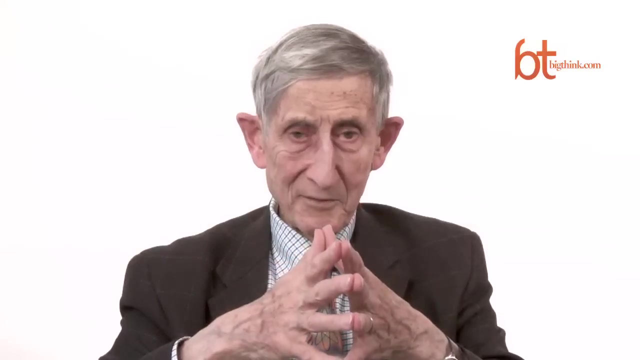 And what we've seen is that the earthquake in Chile was much larger, but the damage actually was smaller, the reason being that Chileans had taken more trouble to build buildings that would resist earthquakes, So it actually helps enormously to strengthen your buildings. Of course, Chile has the advantage. 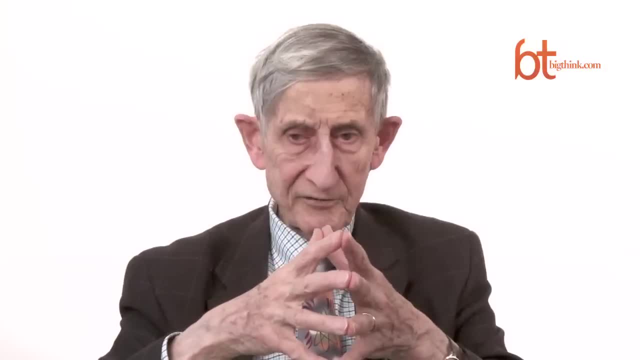 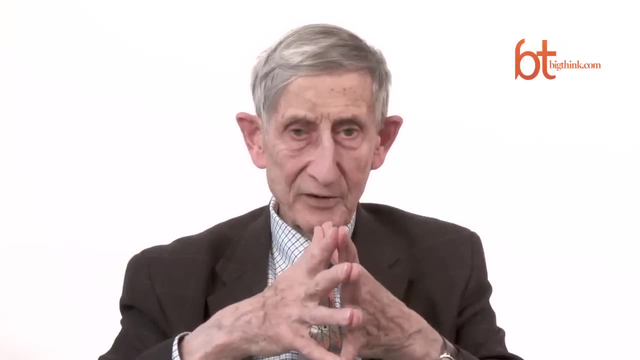 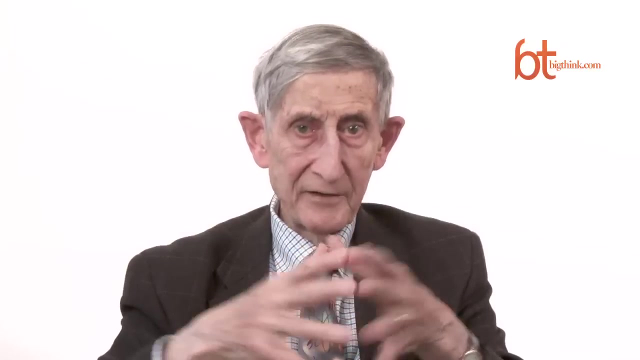 of being a richer country to start with, but it's a dramatic proof of what you can do. You can actually take a natural catastrophe and reduce the damage by a factor of 100 or so just by quite simple measures, just having good building codes. 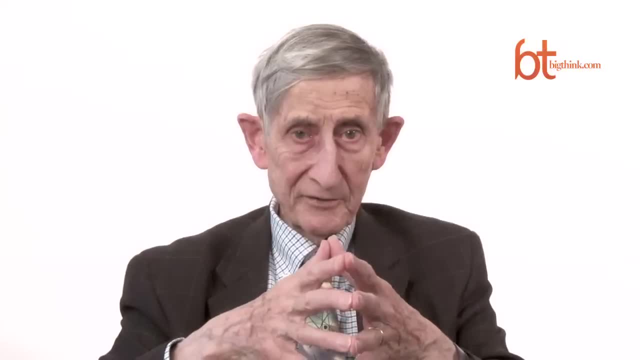 And the same is true of climate. There are all sorts of things we can do in a practical way. It's not only we don't only have to worry about warming, we also have to worry about cooling. It could very well be the climate gets colder, Nobody knows. 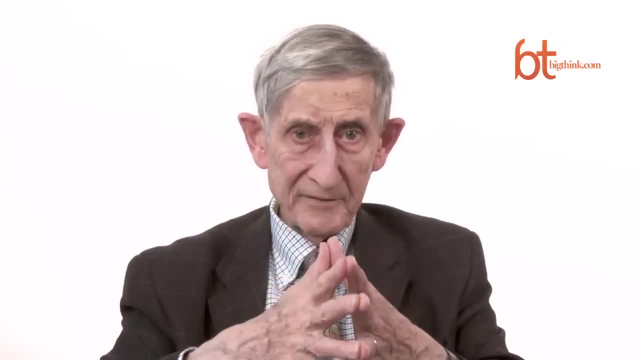 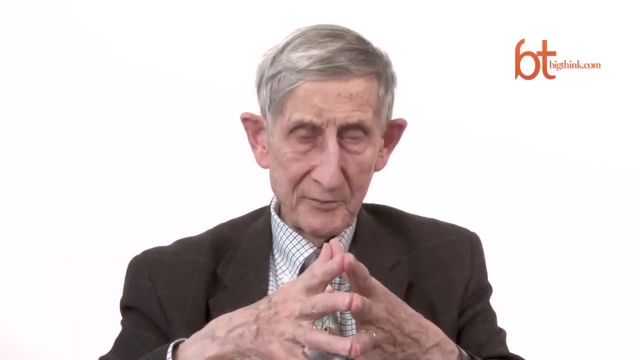 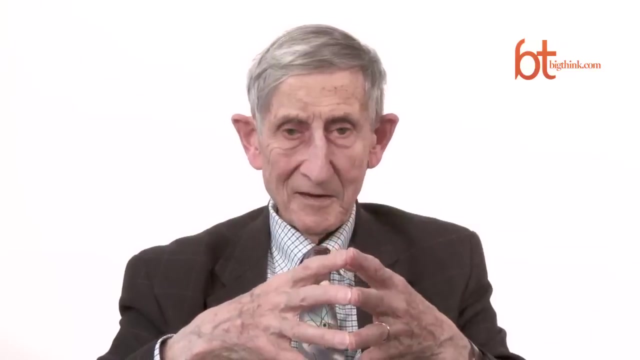 And there are many things we should be doing to prepare for that, and they're not all that expensive. But what I think is absurd, what I disagree with very strongly, is the idea that climate is predictable, that we can do things 100 years in advance, knowing what's going to happen. That's just not the way it is.